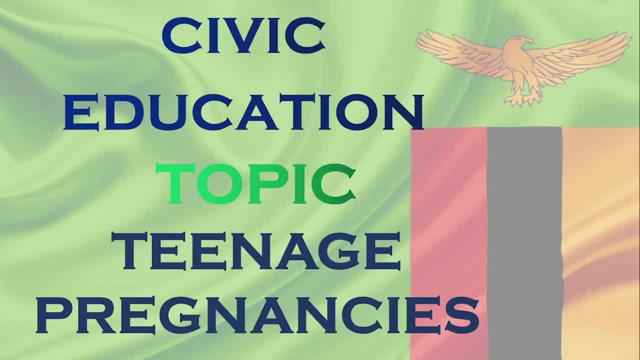 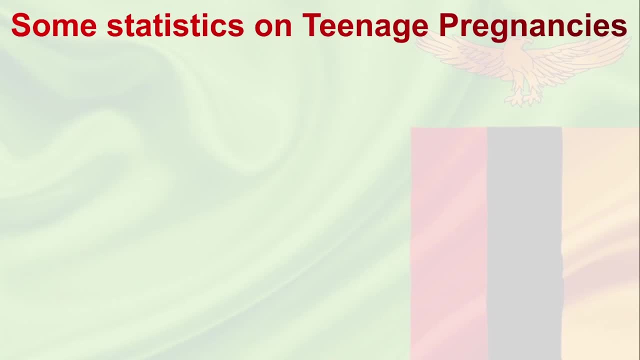 the challenges that young mothers face, or young fathers face, when they have a child at a tender age. So the first thing that we're going to do is we're going to look at some statistics on teenage pregnancies around Zambia. Mostly, we'll concentrate on the eastern side of Zambia because we have 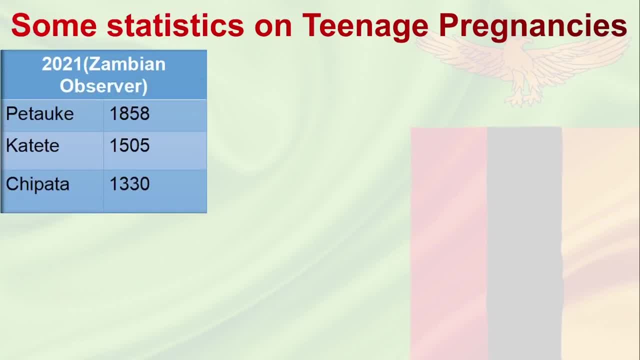 more statistics coming from that side. So the first one that we look at is: according to the Zambian Observer 2021, Petawuke had 1,858 teenage pregnancies, Katete 1,505 and Chipata 1,000.. 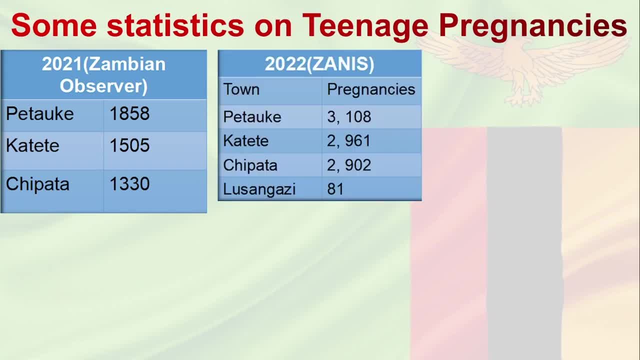 In 2022, Zanis reports that Petawuke, which in the previous year had recorded 1,800, in 2022 had 3,108.. Katete 2,961, followed by Chipata, with 2,902 pregnancies. 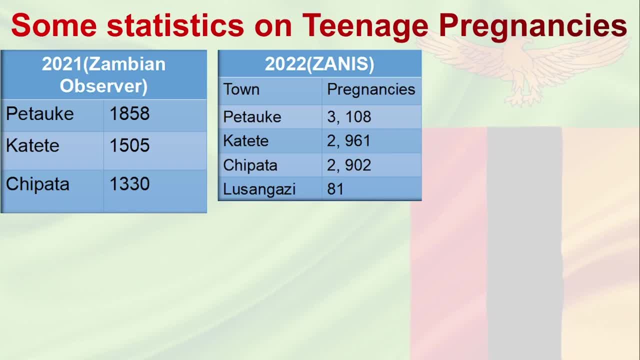 Then we have Lusangazi there, which recorded 81.. In 2023, according to ZNBC, from January up to September, the same Lusangazi, which had 81 in 2022, now had 800 pregnancies and out of those, 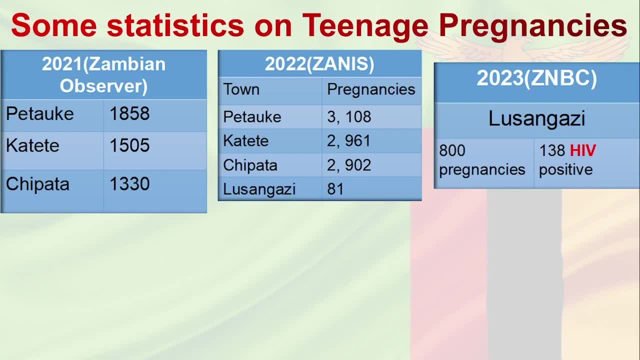 138 tested HIV positive, Again in 2022,. we look at some statistics that are coming from Northwestern. Zanis reports that there were 1,600 pregnancies and among those 100 of them were girls aged between 10 and 14.. So those are some of the statistics. 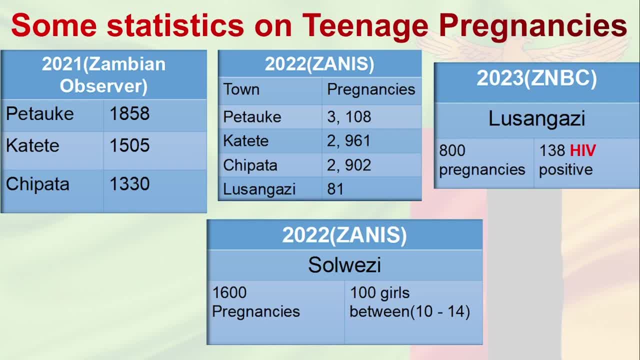 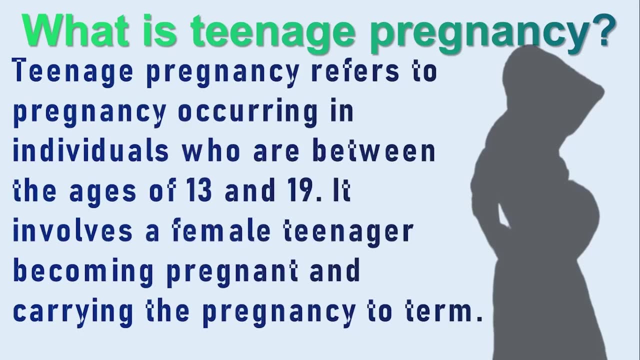 We can research more, read more on some of the statistics from different provinces, different countries, so that we understand the issue that surrounds teenage pregnancies. Now, what is teenage pregnancy? Teenage pregnancies refers to pregnancy occurring in individuals who are between the ages of 13 and 19.. It involves a female teenager becoming 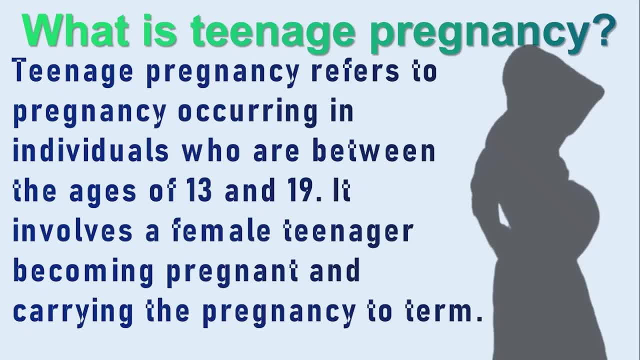 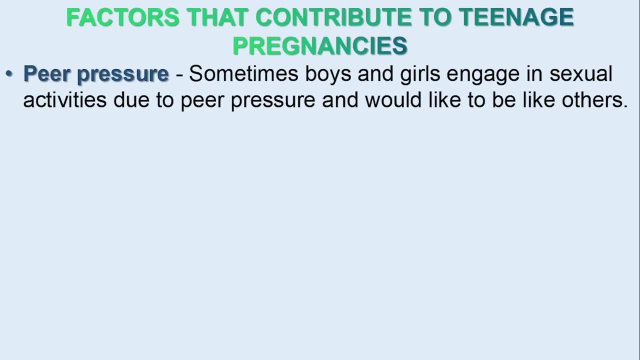 pregnant and carrying the pregnancy to 10 or until they give birth. There are a number of factors that contribute to teenage pregnancies. One: peer pressure. Sometimes you find that the boys and the girls engage in sexual activities due to peer pressure that is coming from their friends, Because their 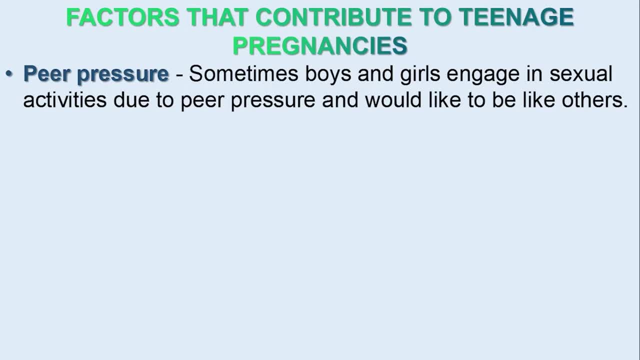 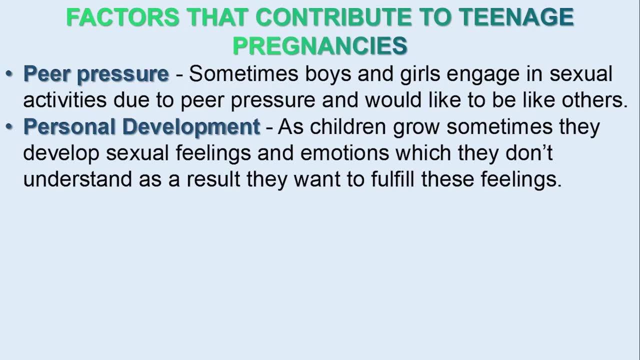 friends are doing this. they also want to encourage their friends to do the same. The second one is personal development. As children grow, sometimes they develop sexual feelings and emotions which they don't really understand and, as a result, they want to fulfill these feelings. 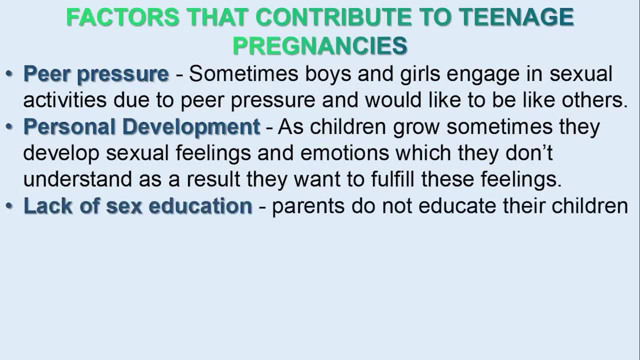 The third point that we have is lack of sex education. Sex education plays a crucial role in empowering teenagers with knowledge about their bodies, relationships and self-practices. Unfortunately, many educational systems have fallen short in providing comprehensive sex education, which leaves most adolescents or teenagers uninformed. 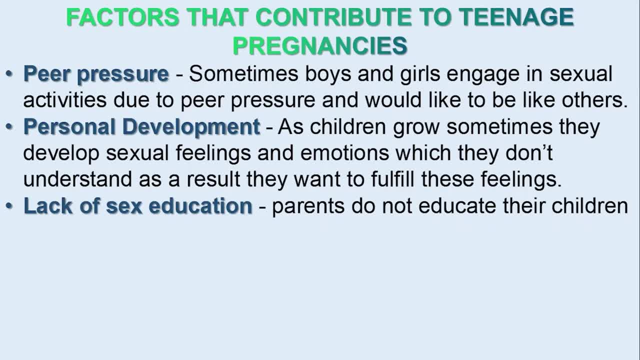 Without proper sex education, teenagers may engage in risky behaviors and make uninformed decisions. The other point is society and media influence. Now, this one mostly. we are talking about the society's influence as well as the media influence, For example, songs or movies that we watch, or even some of the friends that we have that have gone through teenage pregnancy. 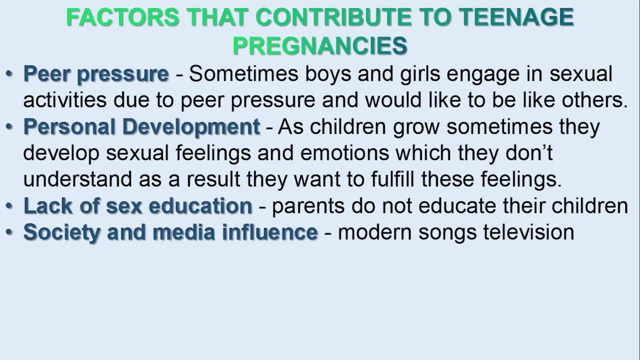 Now societal norms and expectations can heavily influence. Sometimes there is stigma around discussing sexuality openly, which may contribute to a culture of silence and preventing teenagers from seeking guidance or information about the problem. Then, on the media side, here we say we are looking at movies, TV shows and even the social media these days. 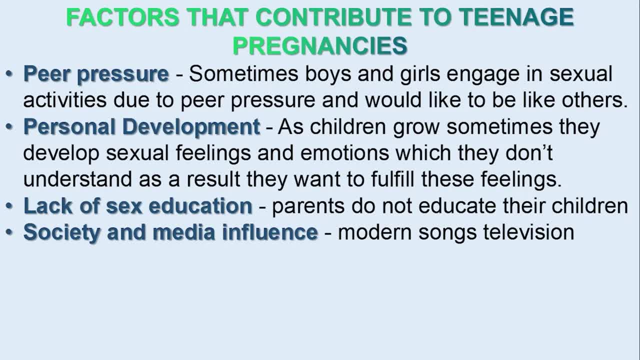 Now you find that often these platforms romanticizes or grammarizes teenage pregnancy. It can create an unrealistic expectation and they are going to downplay the challenges that are associated with early parenthood. The other point is cultural issues. Now girls are married off at early ages and sometimes are not allowed to go to school. 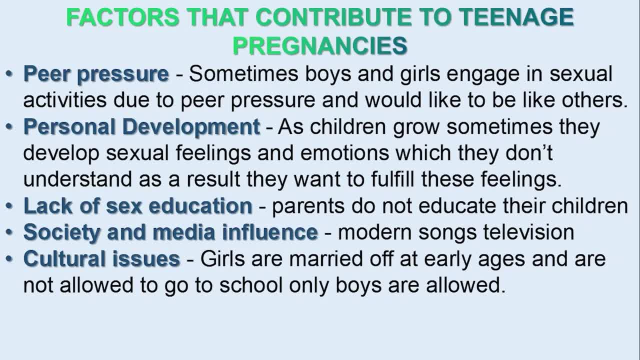 because the parents do not see a point in taking a girl child to school Because in their mind this child is just going to get married And go off with the family of the man, So there is no point in educating her. So they would rather just give her away into marriage and they get the lavola or the bride price that is paid for the girl. 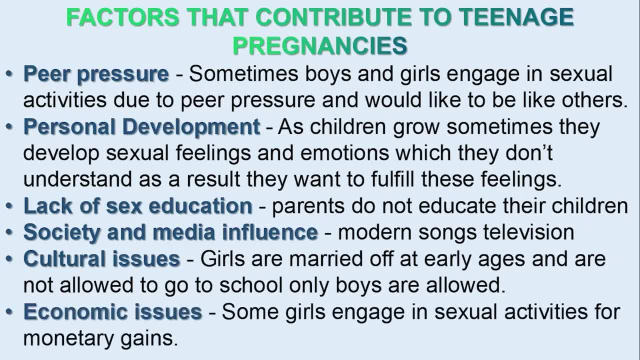 Then the sixth point is economic issues. Some girls engage in sexual activities for monetary gains. You find that some girls will engage themselves in sexual activities so that they can get a little bit of some money. They can use it, They can use at home. 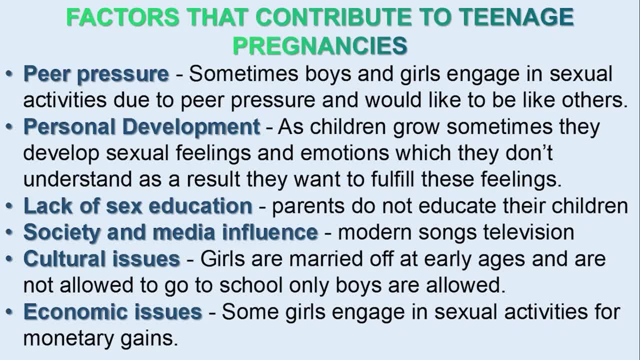 So it's the only way that they find as a way of raising some money so that they can have a meal, While others do this so that they can have the fancy things that their friends are having, like the new cell phones or the new shoes. 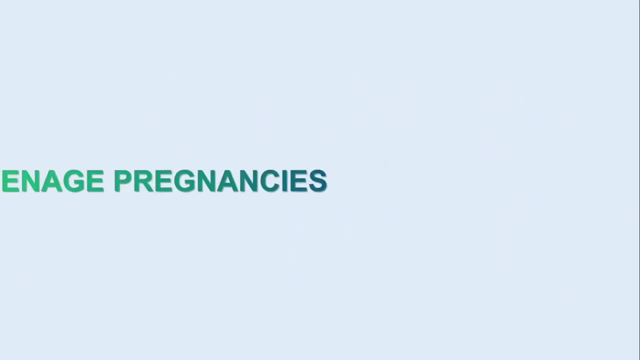 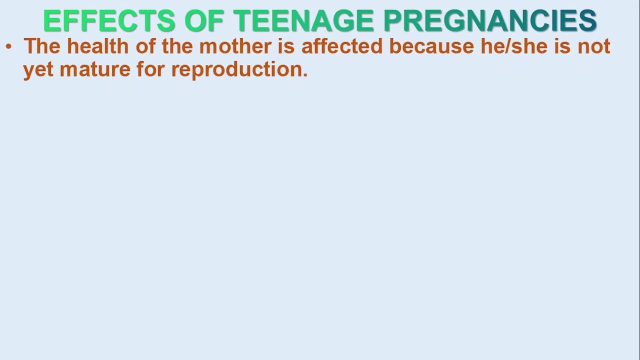 the new outfits that are coming on the market. Now let's look at the effects of teenage pregnancies. One of the effects is that the health of the mother is affected because he or she is not yet mature enough. The mother is not yet mature for reproduction. 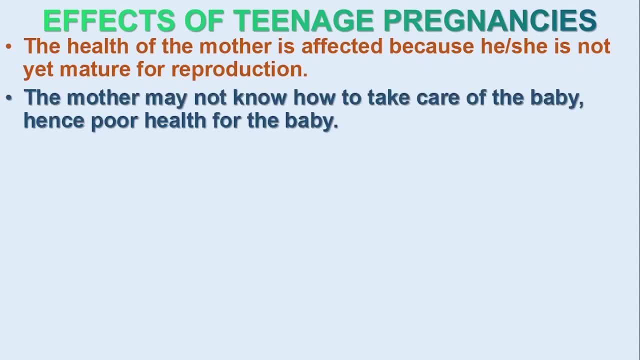 I think that is common sense. Then we also know that the mother may not know how to take care of the baby. Hence the baby is going to face some poor, healthy issues, For example eating. The mother may not know how to feed the child properly. 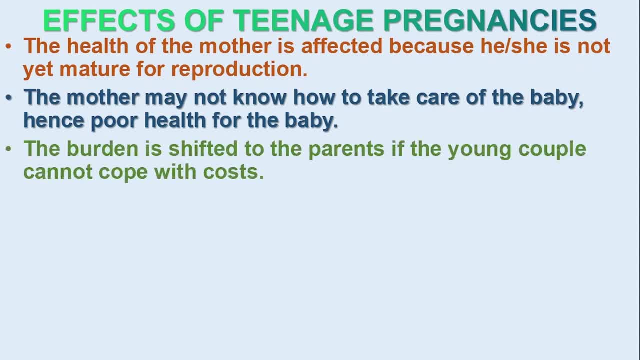 The other point is the burden is shifted mostly to the parents, especially of the girl, if the couple is young and they cannot cope with The costs of taking care of the baby. The other point is child dumping. Now, child dumping refers to the act of abandoning infants or young children in public places, often leaving them without proper care or support. 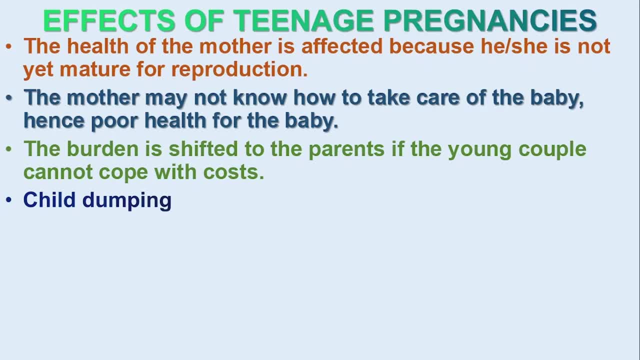 This has serious implications for the well-being of these vulnerable individuals. Children who are subjected to dumping face immediate dangers to their health and safety. They may experience a dog trying to eat them, or even some rats, That is, if they are not found by a good Samaritan. 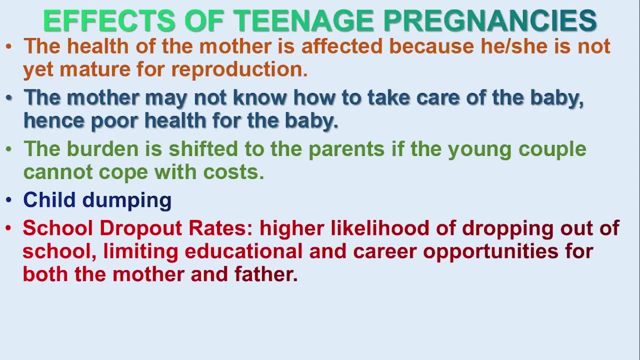 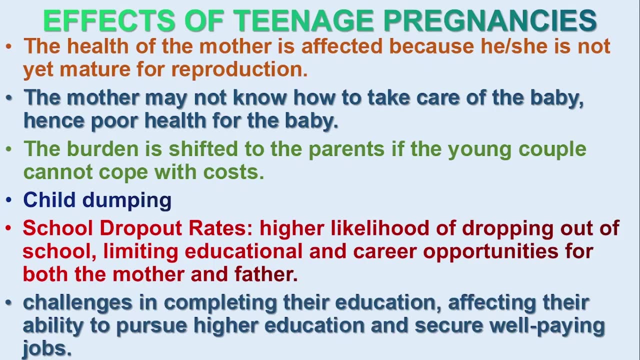 Then the other point is school dropout rates. It refers to a higher likelihood of dropping out of school, limiting educational and career opportunities for both the mother and the father. And the last point is the challenges in completing education, Which affects the ability for the young mother and the young father to pursue higher education and secure well-paying jobs. 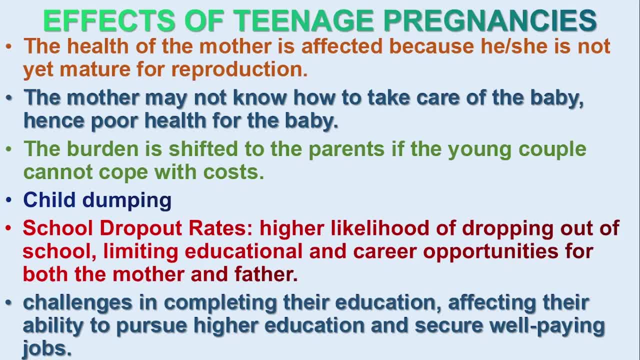 Because they're busy at home taking care of this child, So you find that they will not have enough time to explore and discover themselves and grow their own career. Now, how can we prevent teenage pregnancies? We'll discuss some of the things that we can do to prevent teenage pregnancies. 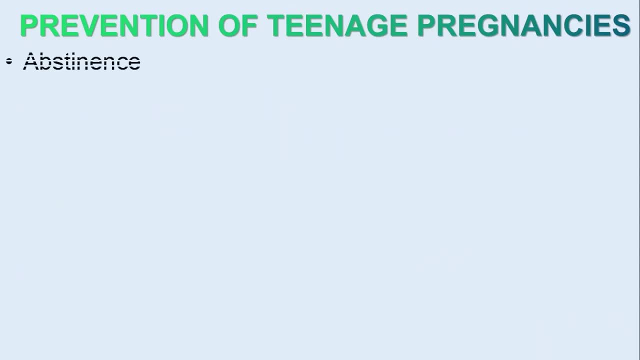 So the first one is we can abstain, stay away from sex. The other thing that we can do is avoid bad company. The other thing that we can do is we can learn life skills and also do some decision making programs Which can help improve our lives and help us make better decisions. 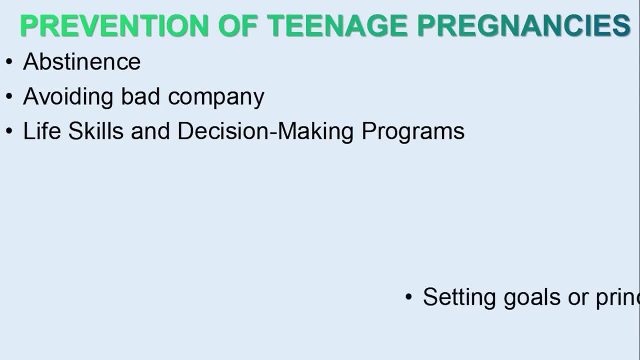 Especially concerning sexual activities. We can also set goals or principles, To say: this is what I want and I'm going to achieve it. I'm not going to engage myself in these activities until I am at a certain age or until I have achieved certain goals. 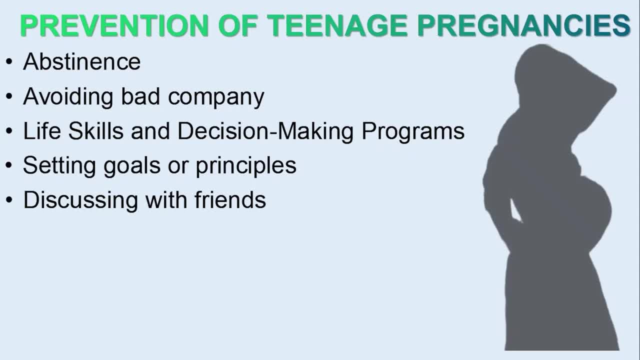 The other thing that we can do is we can discuss with friends about the challenges of teenage pregnancies. Talk about this thing openly with friends. Consult from people who have gone through these things. It's going to help us in preventing teenage pregnancies. The other thing we can do is we can avoid alcohol and drugs. 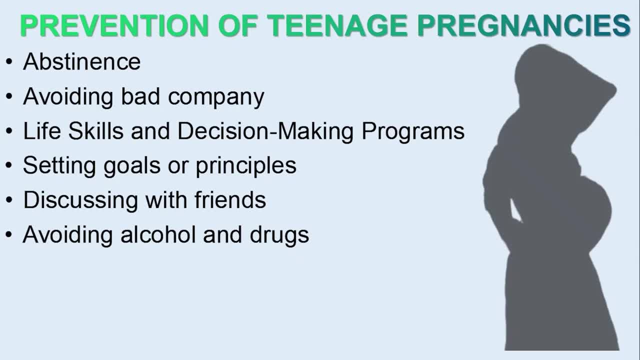 These substances lead young girls and boys to engage in sexual activities after they have taken alcohol or have taken drugs, And they may find themselves being pregnant at a tender age. So let's avoid drinking and engaging in substance abuse. Let's also try to resist peer pressure. 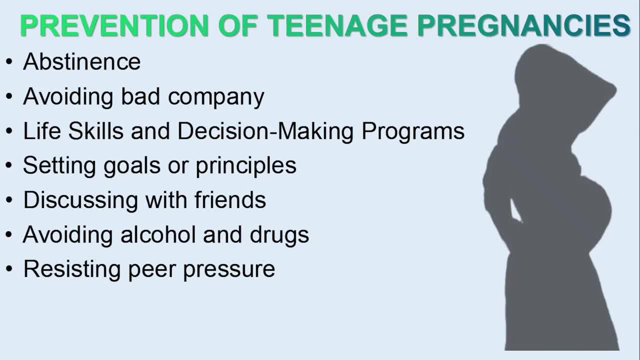 Peer pressure is something that, if we're not very careful, can lead us into things that are not pleasing and may affect our future lives. Then we can also uphold the good morals and values that we have been taught at home. Our guardians, our parents, our aunties, uncles, have told us to look after ourselves.